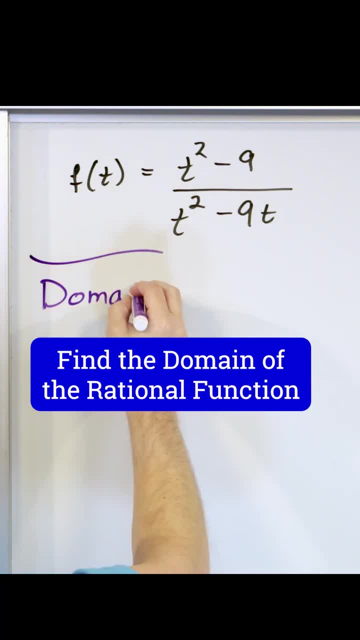 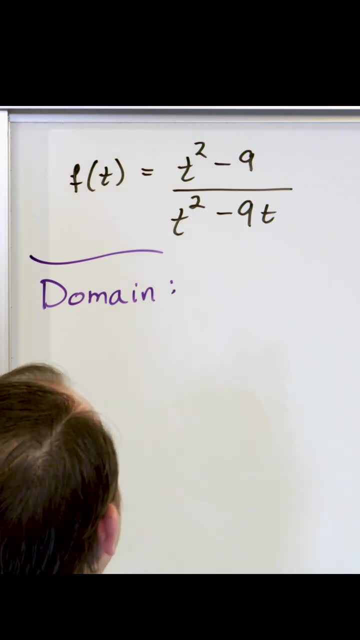 So, to figure out the domain of this function, what do we do? We set the denominator equal to zero, because those are going to be the, basically the, they're going to be the values of t that aren't even allowed to go into this function because they blow the whole function up to. 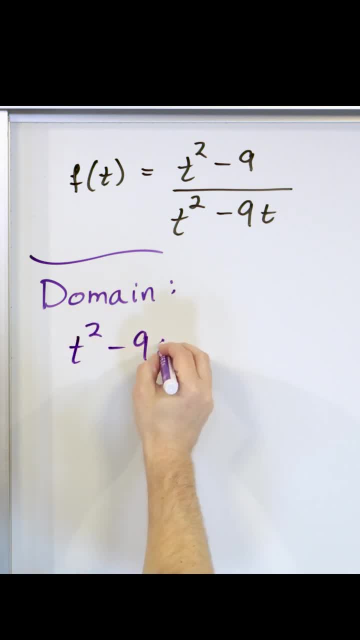 infinity. So we say t squared minus nine times t is equal to zero And we have to solve this equation. So we can pull out a t Inside, we'll have t minus nine equal to zero. So we have t can be equal to zero and this can also be equal to zero. So we have t is equal to zero and also. 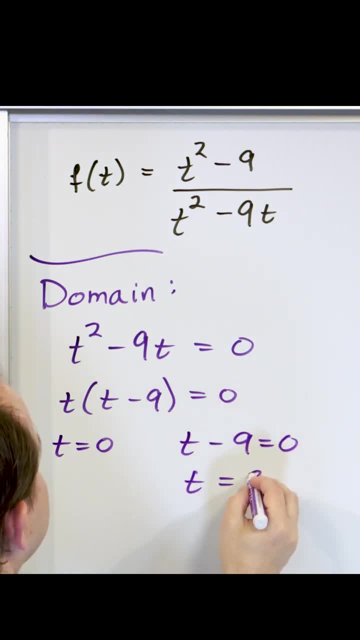 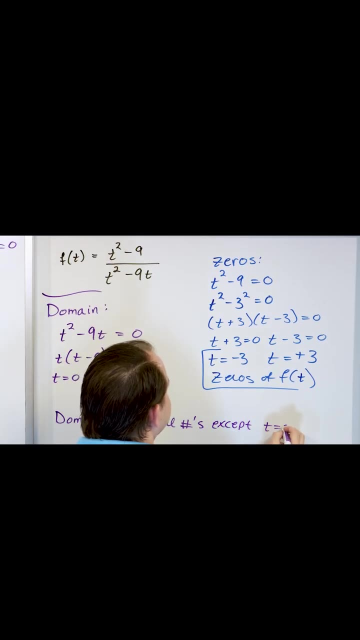 t minus nine can equal zero, which means that t can be equal to nine. So what it means is that two different values of t cause problems for this function. So the domain is all real numbers. That means all negative and positive numbers, except for t equals zero and t is equal to nine. This 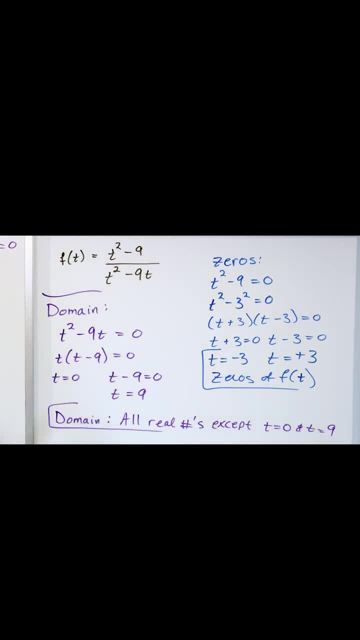 is what you would circle for the domain. All real numbers except for t is equal to zero and t is equal to nine. Learn anything at mathandsciencecom. 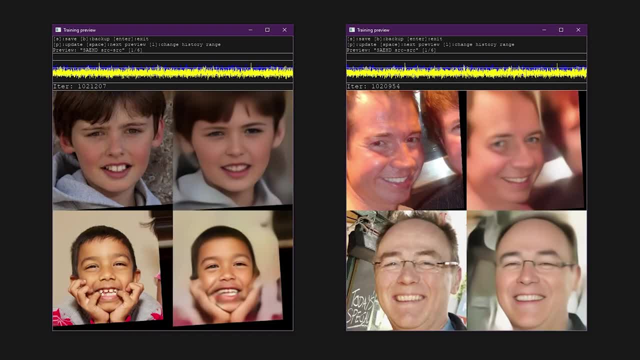 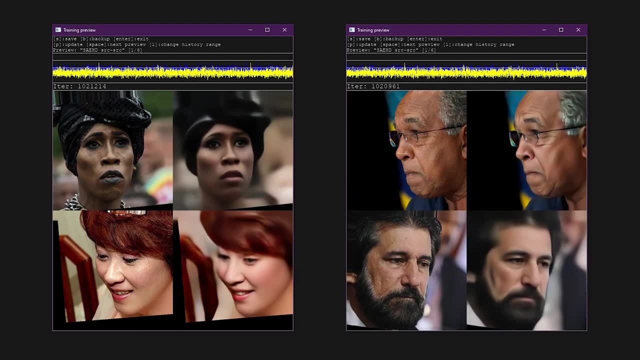 Today, I'm going to show you how to speed up the deepfake process by creating pre-trained models. This video will also serve as a primer for those who are unfamiliar with the DeepFaceLab training settings. A pre-trained model is created with a face set consisting of thousands of images. 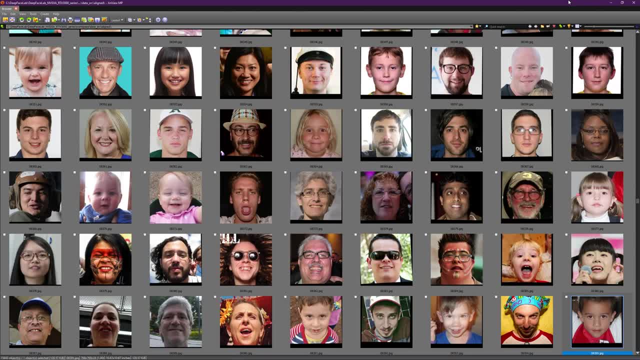 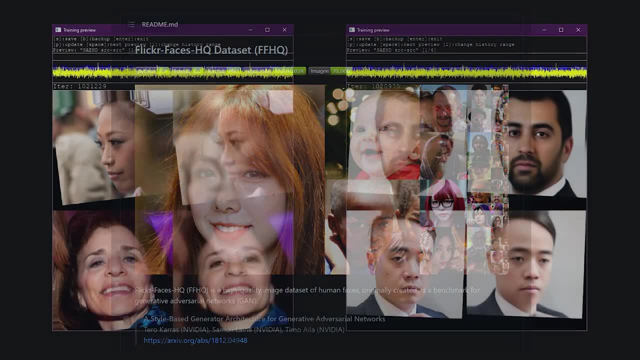 with a wide variety of angles, facial expressions, color and lighting conditions. DeepFaceLab includes such a face set derived from the Flickr Faces HQ dataset. To get started pre-training a model, the only thing you need is DeepFaceLab. No other images or videos are required. 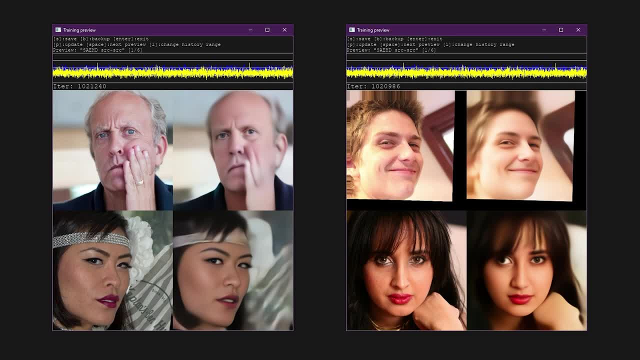 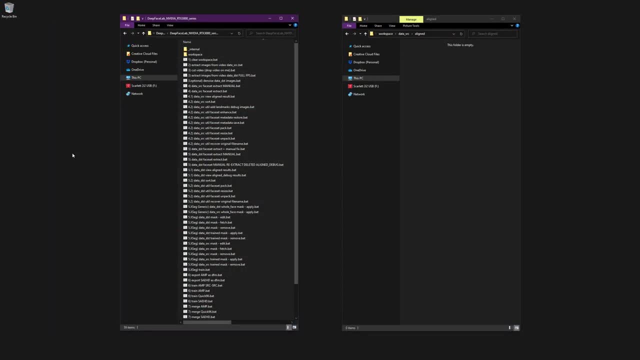 Since the Quick96 and AMP models do not offer a pre-training option, this video will focus on the SAE HD Trainer, which is the standard for most deepfakes. First off, if you want to view, modify or replace the default pre-trained face set,